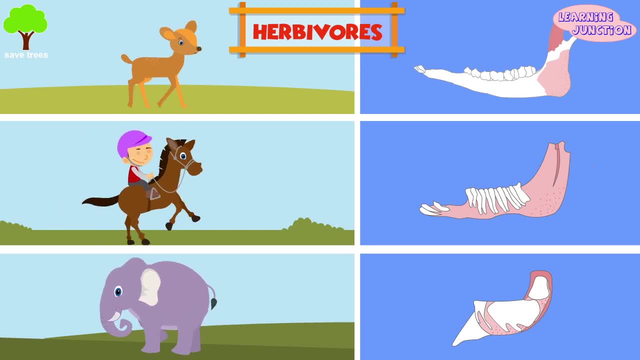 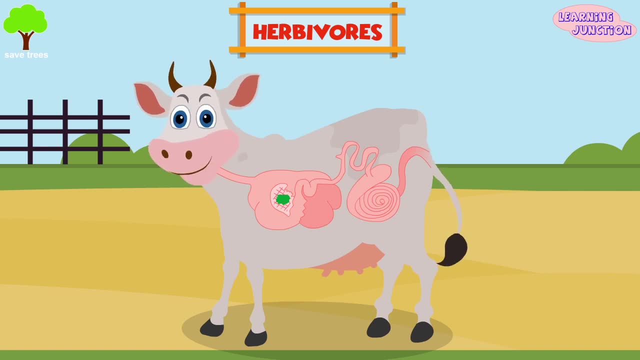 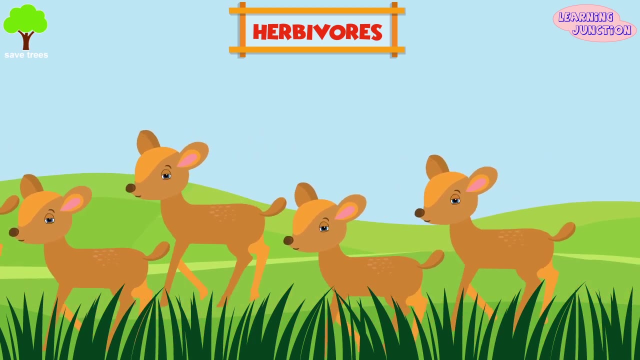 adapted to easily grind vegetable tissues. These herbivores have evolved different type of digestive systems capable of handling large amounts of plant material. They generally have eyes on the side of their head, which allows them to have a wider field of vision, Thus allowing them to see all the way. 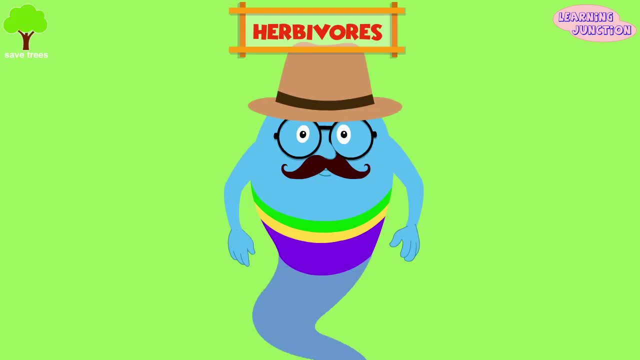 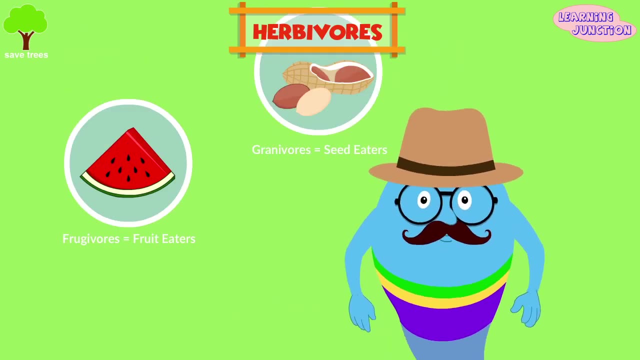 around with a 35-degree angle. Herbivores eat a variety of vegetables, including without even moving their heads. Herbivores can be further classified into frugivores, meaning the fruit eaters, granivores or the seed eaters. 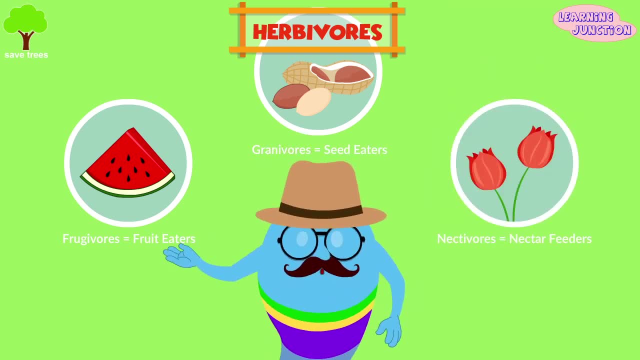 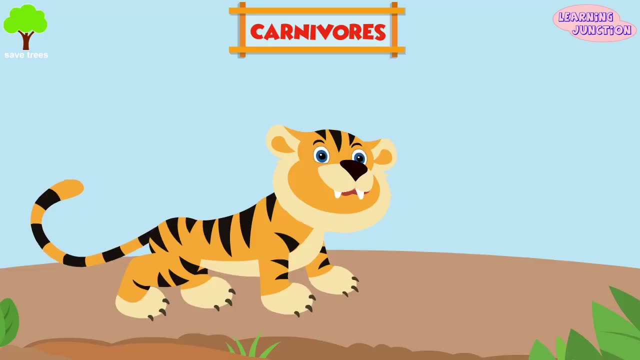 nectivores means nectar feeders and folivores meaning the leaf eaters. Now let's study about the carnivores. A carnivorous animal consumes animal tissue, flesh, organs and bone in order to feed and gain energy. 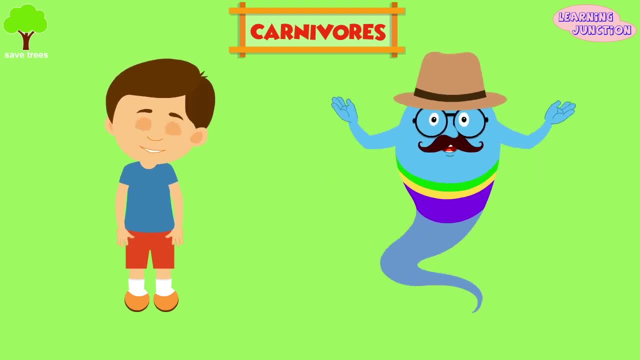 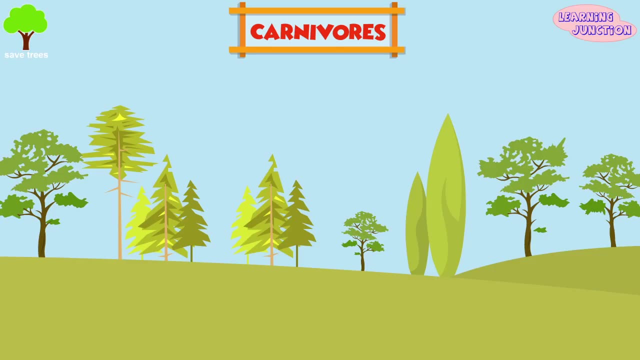 Common characteristics include speed, strength and keen senses for hunting, as well as claws and teeth for tearing and capturing prey. Many of them, like leopards, lions, etc. chase their prey and kill it with their sharp and pointed teeth. 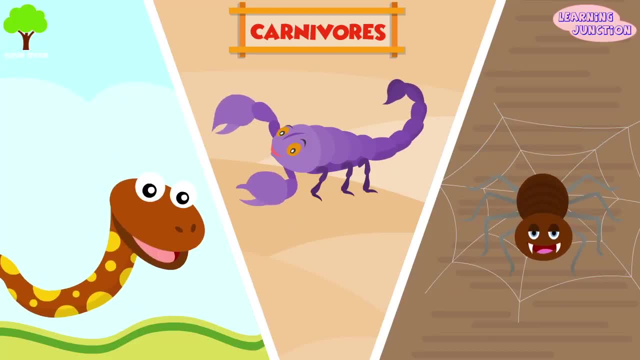 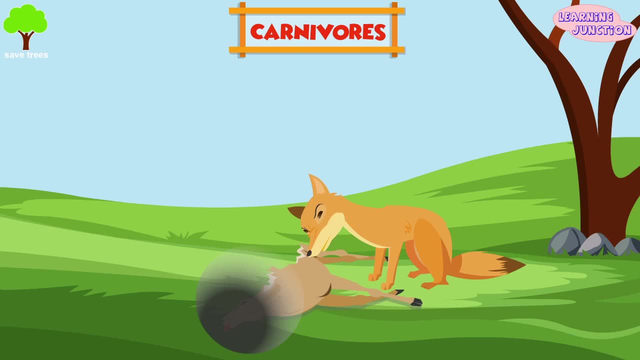 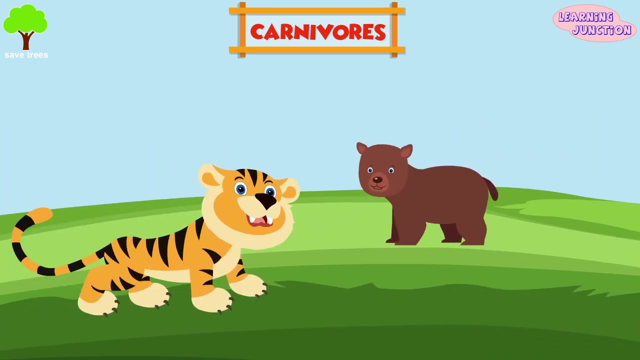 Some carnivores, including snakes, scorpions and spiders, inject venom to overpower their victims. Other carnivores, like jackals and raccoons, do not kill their prey but instead eat the flesh of dead animals. Animal blood and flesh contains lots of energy. 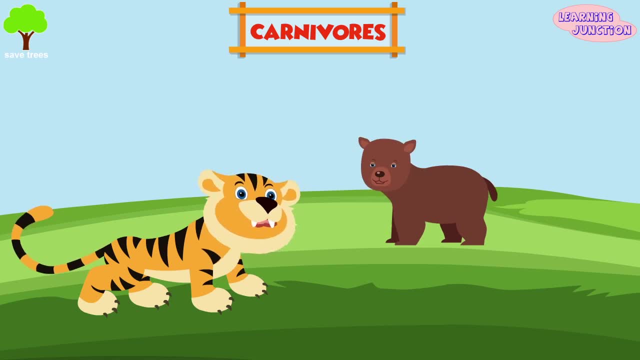 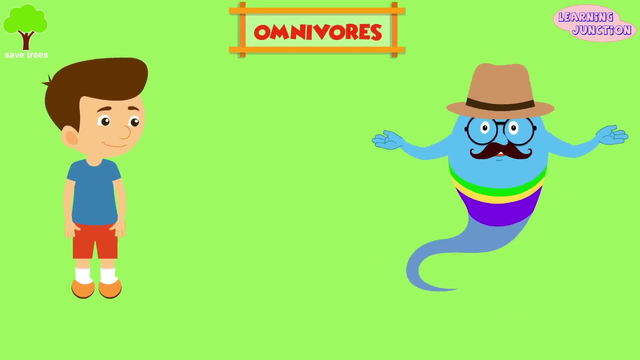 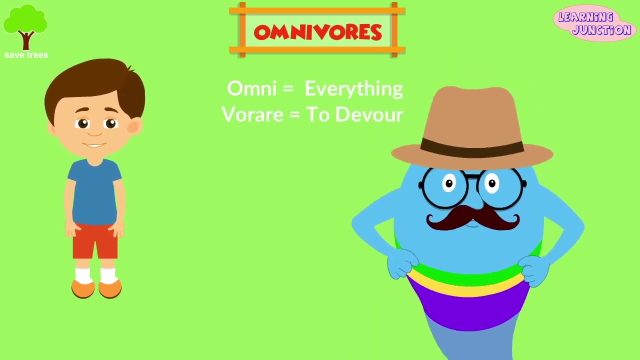 so many carnivores can survive for a long time between meals. And now the omnivorous animals. Omnivores comes from the Latin word omni, meaning everything, and vorere, meaning to devour, So an omnivore will eat pretty much anything in sight. 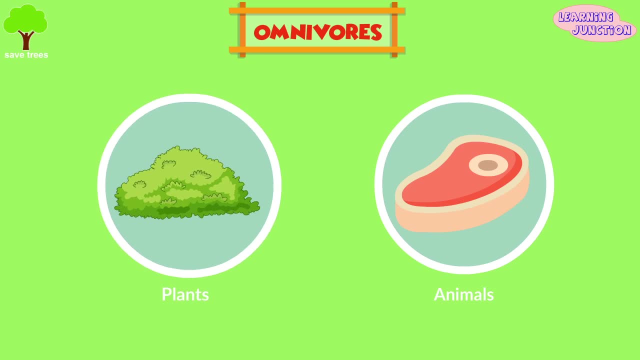 An omnivore is an animal that is able to eat anything in sight. An omnivore is an animal that is able to eat anything in sight. An omnivore is an animal that eats both plants and animals, which may include eggs, insects, algae and fungi. 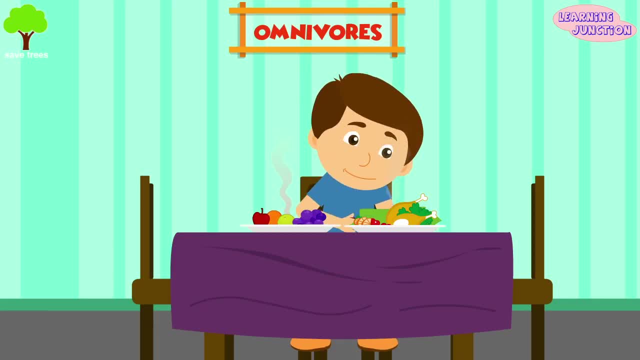 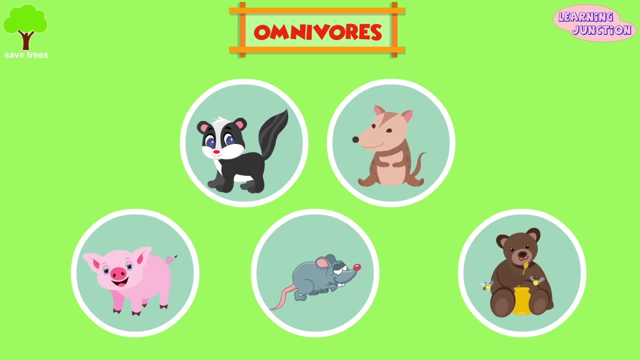 Humans are genetically designed to be omnivores. Some common omnivores include possums, skunks, pigs, rats and most bear species. Hmm, some reptiles such as lizards and turtles are also omnivorous.